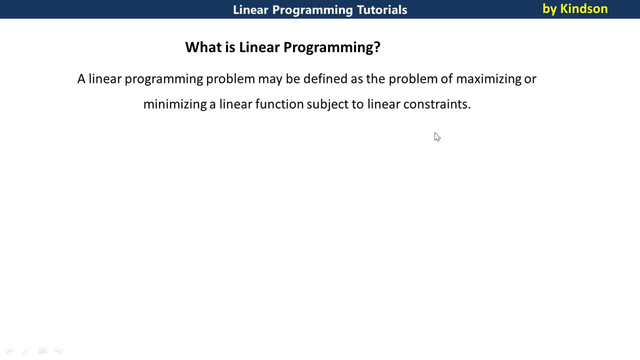 A little bit of history about linear programming. it actually started in the mid 20th century during the Second World War, when engineers have to find a way to maximize resources or maybe minimize the time it takes to move equipment from one location to another. So it's actually a way to solve real life problems. 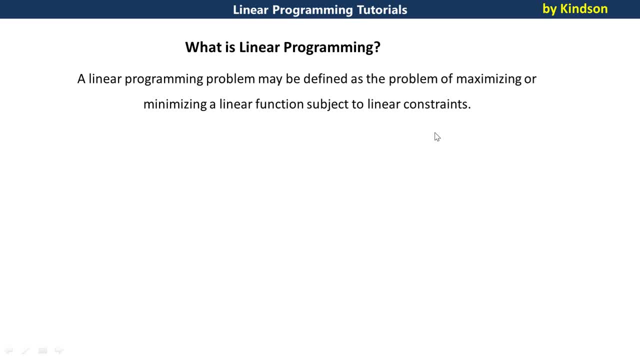 And that is why most of the time you see expressions like linear programming. So once you can break a problem down to linear programming, a proper problem, then you can actually apply the principles of linear programming to actually solve this problem. So let's see how it works. 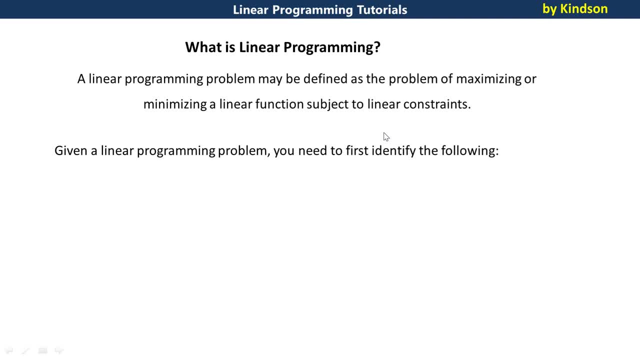 So, given a linear programming problem, how do you actually solve a linear programming problem In the first place? what is a linear programming problem? We've identified it. That is a problem that You need to solve based based on certain constraints or constraints, and also know that it has to be either maximizing or maximizing the functions has to be linear, not polynomial function, or not nonlinear function. 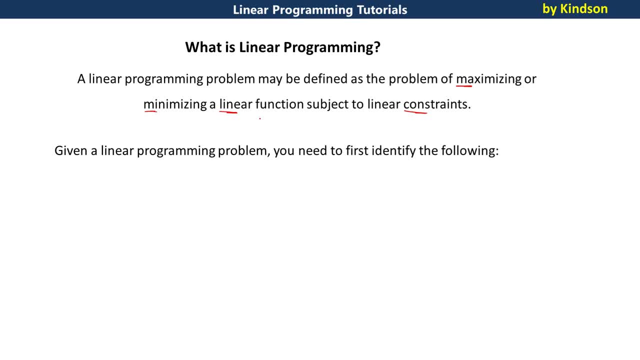 And then you have to solve this problem. So, given a problem, The first step in solving a linear programming problem is to identify the following four items. One of them is the cost function. So what is a cost function? The cost function is the function. 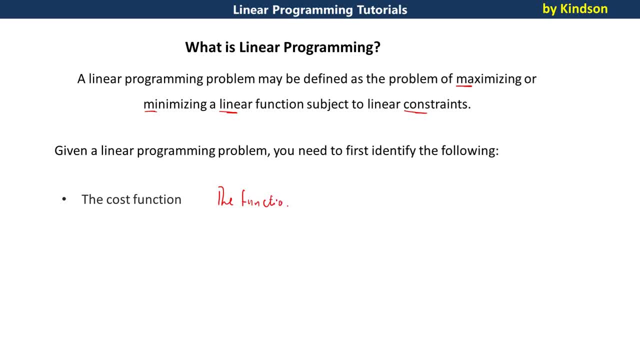 The function you need to minimize or maximize. The function you need To minimize Or maximize. The next thing you need to figure out is the objective of the problem. Are you trying to minimize or are you trying to maximize? I can actually write it out. 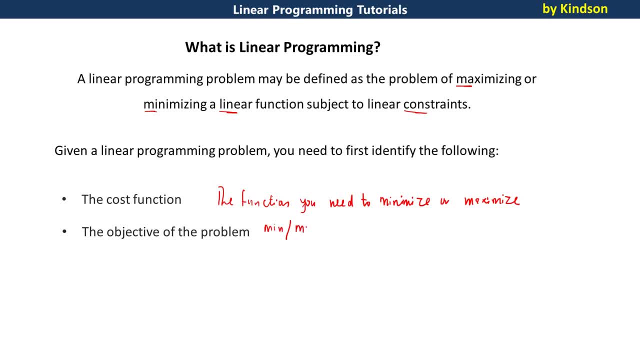 So are you trying to minimize or maximize? So in case of minimizing, it has to be less than or equal to Most of the time, that is what you see. And in case of maximizing, it has to be greater than or equal. 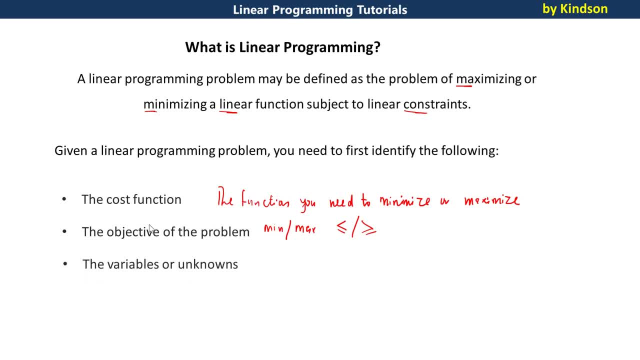 The next thing you need to identify is the variables, or the unknowns. So you need to identify the variables. Most times these variables are not given explicitly, So you need to identify them and assign them: Maybe X1,, X2, X3, or A, B, C, D or X, Y, Z. 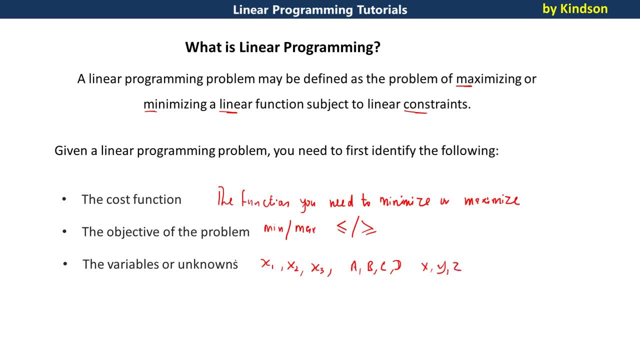 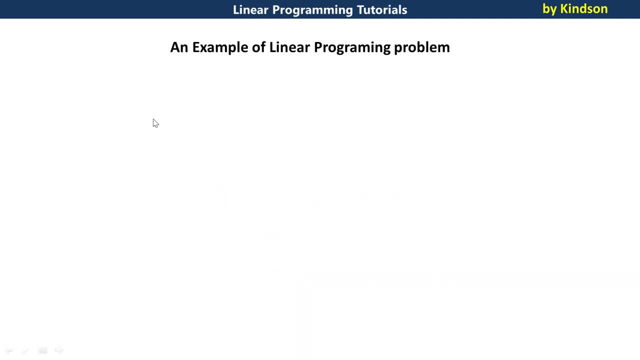 And stuff like that. So you need to identify the variables and assign them certain letters or symbols, And then you need to identify the constraints To make this come alive. let's take a typical example. So let's take an example of a linear programming problem and identify these items that we've mentioned. 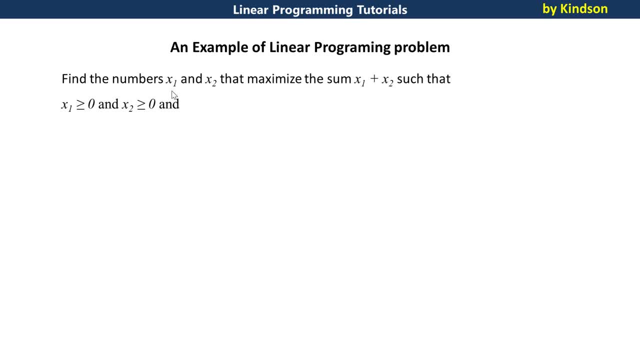 So the problem goes this way: Find the numbers X1 and X2.. That maximize the sum X1 plus X2, such that X1 is greater than or equal to 0 and X2 is greater than or equal to 0. So, and X1 plus 2X2 is less than or equal to 4.. 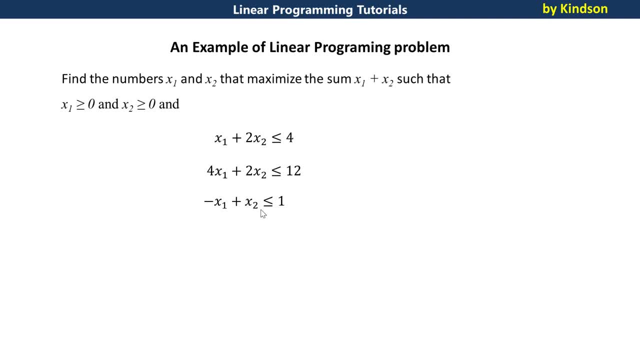 4X1 plus 2X2 is less than or equal to 12.. Minus X1 plus X2 is less than or equal to 1.. So this actually is how linear programming works. So, no matter how complicated, It comes down to all of these. 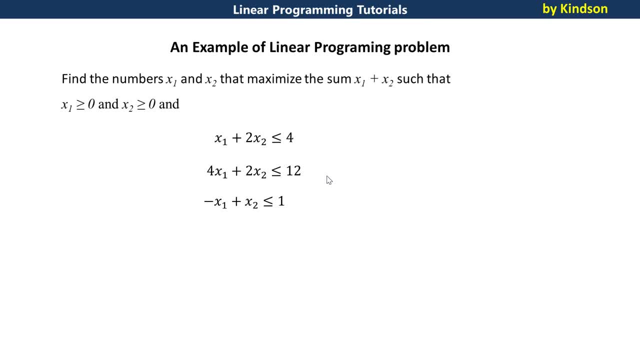 You need to break it down into this. So the only difference is that there may be more than two variables. In this case, we have X1, X2.. There may be more constraints, but everything is actually the same. Just like we mentioned, we need to identify these four functions, these four items. 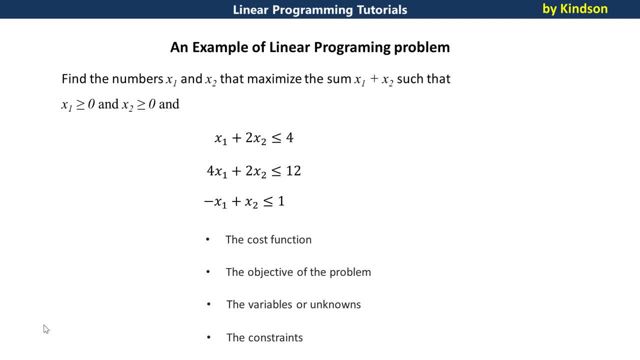 And once you've identified these four items, the problem is actually on the way to being solved. So what is, What is the cost function? in this case, We say: the cost function is a function you need to minimize or maximize. The problem may declare that we need to maximize this. 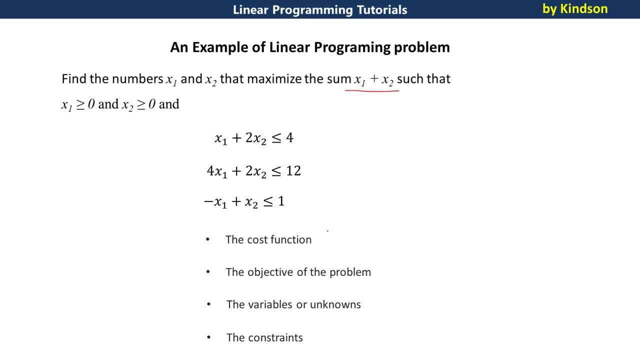 So the cost function, let's say, let's call it, Let's call it: the cost function function of X1 and X2 is X1 plus X2.. So this is our cost function. What is the objective of the problem? 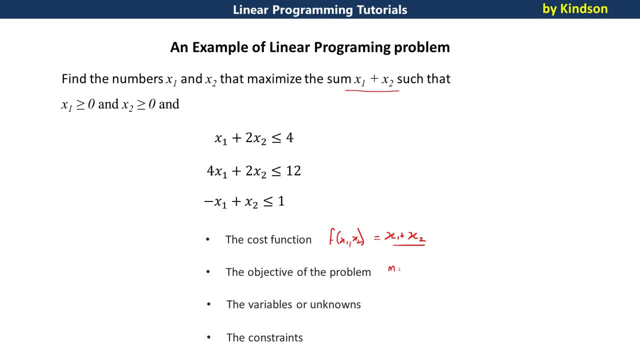 The objective of the problem is to what Is to maximize X1 plus X2.. Right, Good. So if you have some challenges on following, you can just pause the video or you can just make a comment and let me know in the comment box. 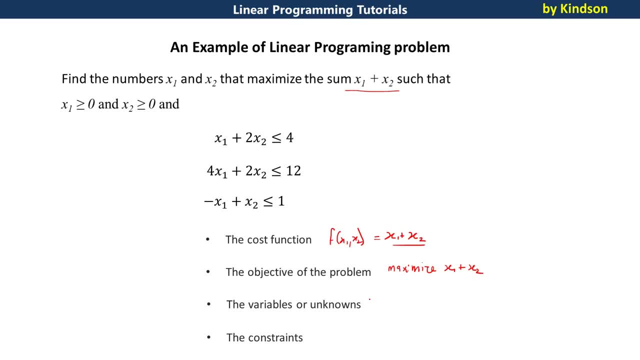 What are the variables? The variables are, Yeah, X1. And X2.. Is there anyone I'm missing? now? I think that these are just the two variables that we have out there. Okay, So what else do we have? We have the constraints. 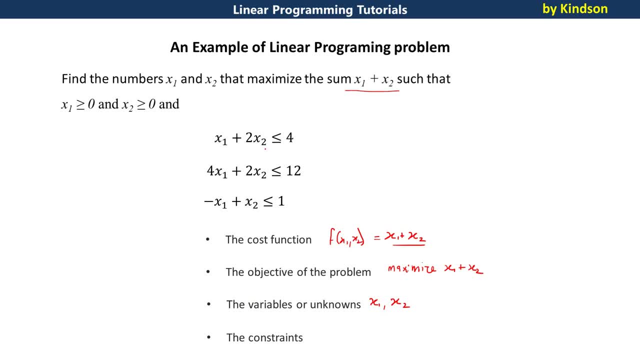 Okay, What are the constraints? The constraints are: 1. Let's call it C1, C2, C3.. C4. C5.. So we have five constraints. We have these five constraints, five constraints, five Cs, These two constraints, I'll tell you: C4 and C5. 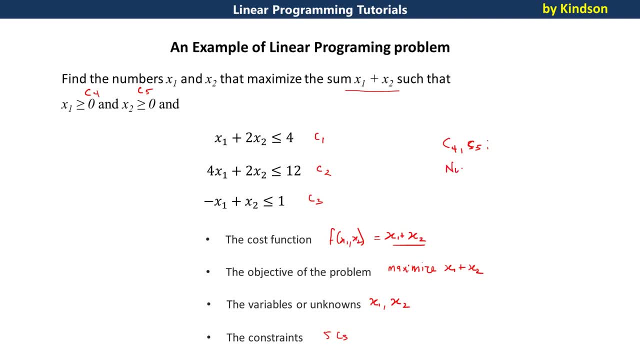 Yeah, They are special constraints and they are called non-negativity constraints. Non-negativity constraints, So for most problems you will, You will always see these constraints for most of the problem, in addition to other constraints. So this is how to break down a linear programming problem. 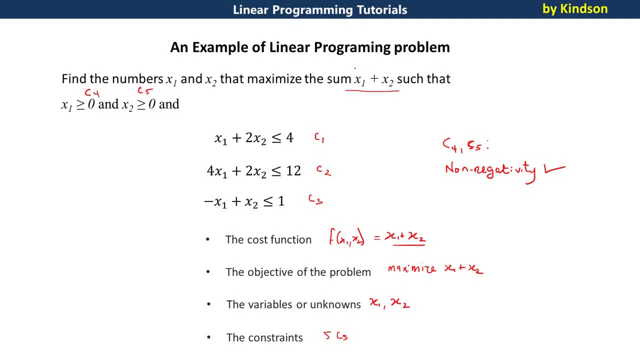 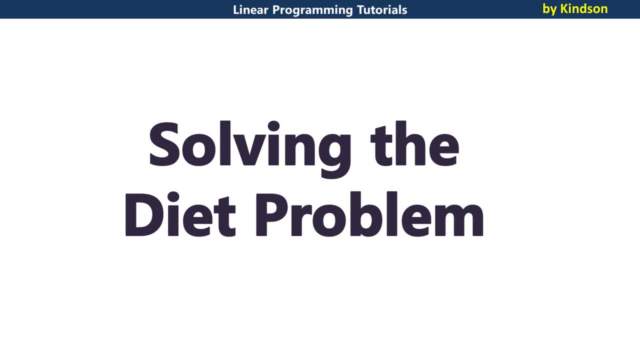